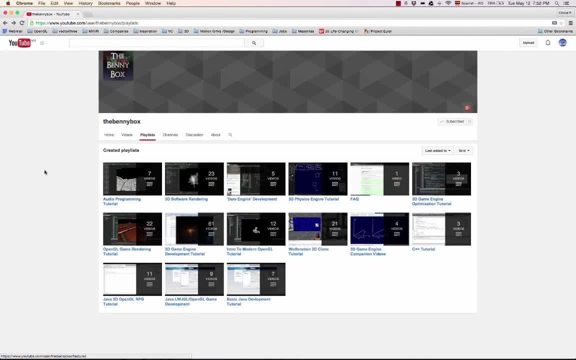 It's called the Benny Box. Here it is. As you can see, it has a lot, tons of great tutorials on 3D game engines, OpenGL, programming and, you know, like computer graphics, It even has a Wolfenstein clone, so it's actually pretty fun. 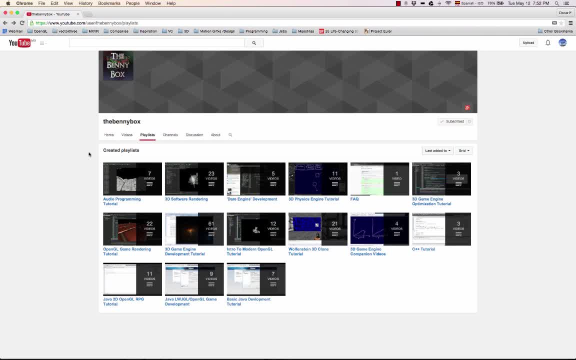 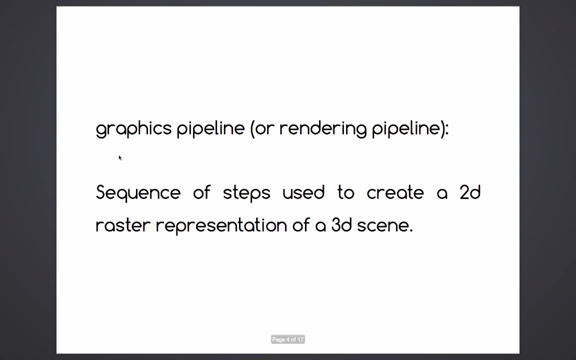 The Benny Box. it, I mean it- has helped me a lot, so it's recommended to you guys interested in computer graphics. So what does graphic pipeline is? I mean at a the very the most common definition is: 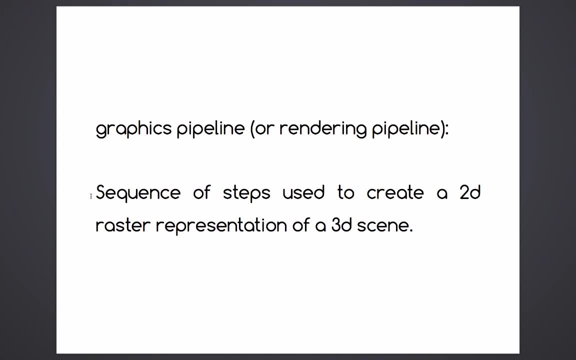 SSL. SSL is a sequence of steps used to create a 2D raster representation of a 3D scene. Plainly speaking, it's: how does the accelerated hardware means the GPU conveys, to port your 3D scene into your monitor, into your screen? 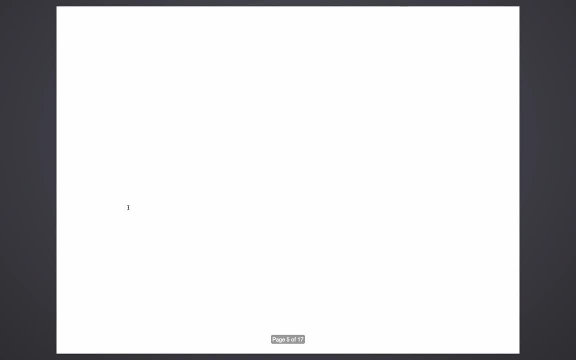 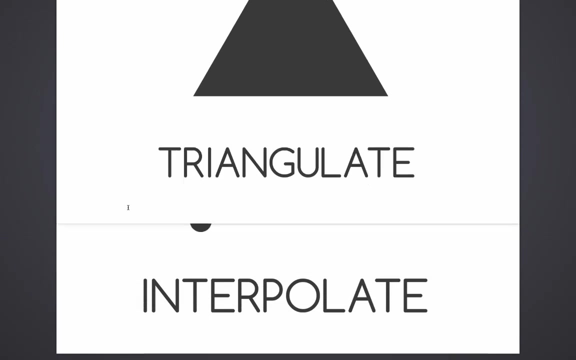 Let's see. I'm going to try to simplify in three steps. what does the GPU? what does the hardware does? The pipeline mainly does three things. First of all, it triangulates the data. It converts everything into triangles, It interpolates between vertices. 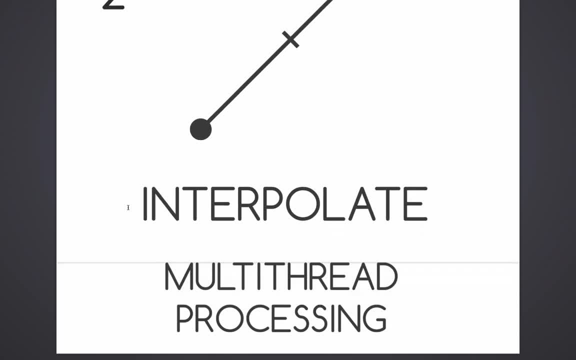 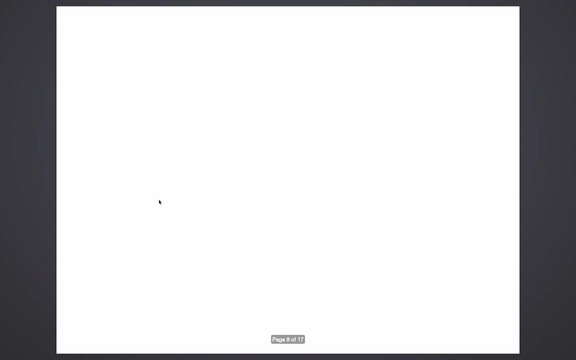 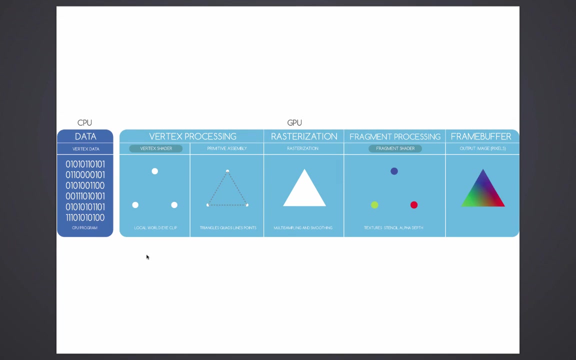 Vertexes, I'm sorry, And It does as it does all this in a multi-threading environment, meaning that it's taking a lot of processes at the same time Means I mean a lot like millions. So okay, let's take a look, a more in-depth look, about the whole graphics pipeline. 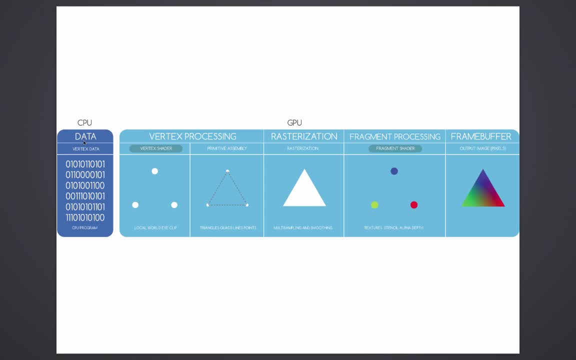 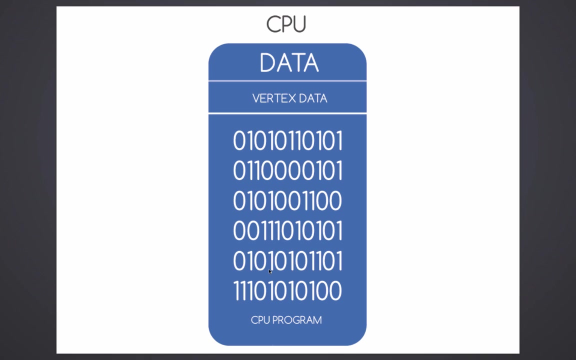 So This is it. It comes from the GPU to the monitor. I'm not sure why I didn't get the label here, but So yeah, The first thing I want to talk about is data. Your graphics pipeline is going to take data. 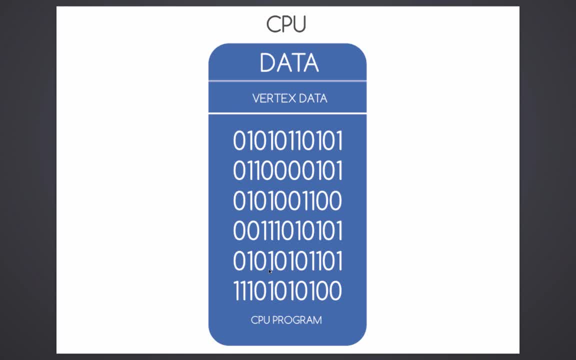 As far as the CPU is concerned, it's just pure 0 and 1 binary data. It could be anything. It could be an application, It could be an operative system, It could be a Word document. It could be anything, For example, models, images, textures, whatever. 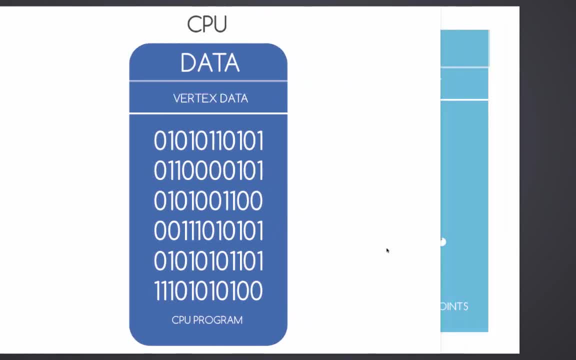 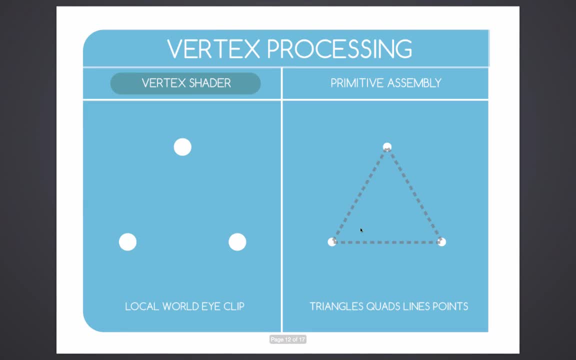 So if that data makes sense, we're going to pass it on. We're going to process that data into something called the vertex processing. This step is going to take that data and analyze it and process it And if that makes sense, it's going to take the input of the vertex shader and create these little points in 3D space called vertexes. 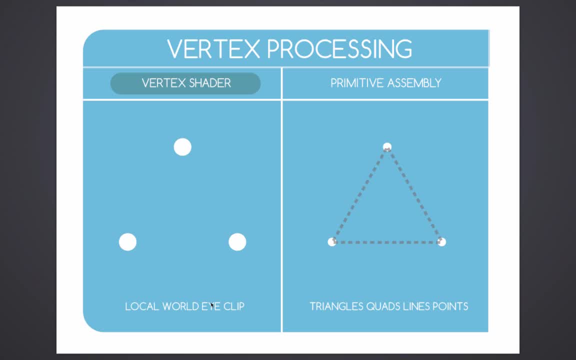 Here we're going to establish our clipping range, our eye projection, our world projection, yeah, our world matrixes, and see where our vertexes are positioned in the 3D space, After the points have been processed and merged with the vertex shader. 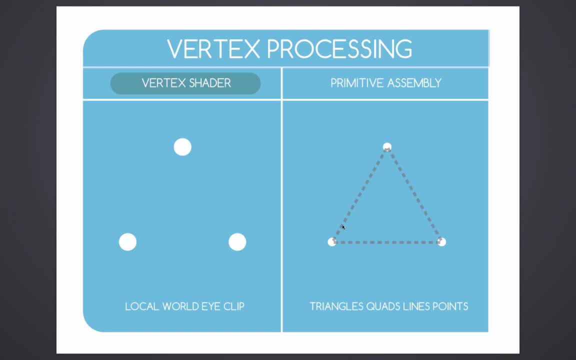 we're going to go to the primitive assembly. This step is mostly ignored, because the next step is where we're going to connect those dots into triangles. The GPU is going to try to connect them And this primitive assembly is a pre-calculation of triangles, quads, lines or points. 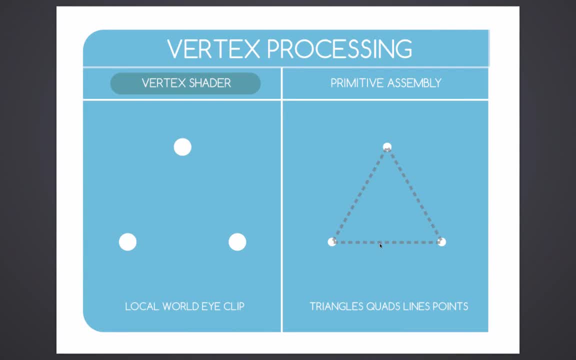 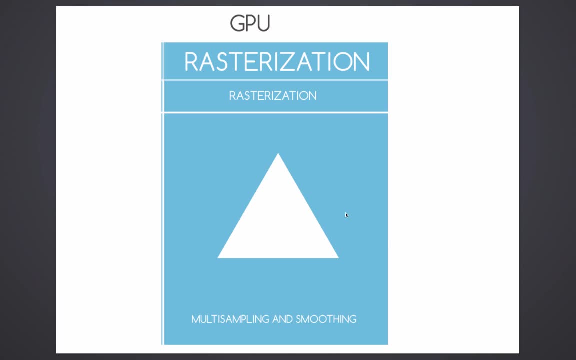 So the next step, the step where the points are connected, it's called rasterization. Rasterization- I'm so sorry It's a long word. Nothing to be afraid of, It's just a really simple step where our 3D calculation 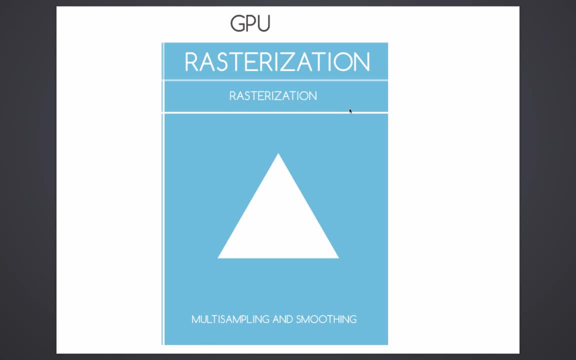 of vertices in the 3D space is converted into a 2D raster. You saw that on the first slide's definition: A 2D raster, meaning we have now a set of pixels And now the GPU is going to work with pixels. 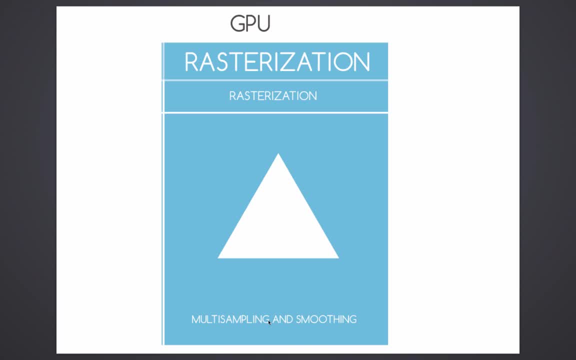 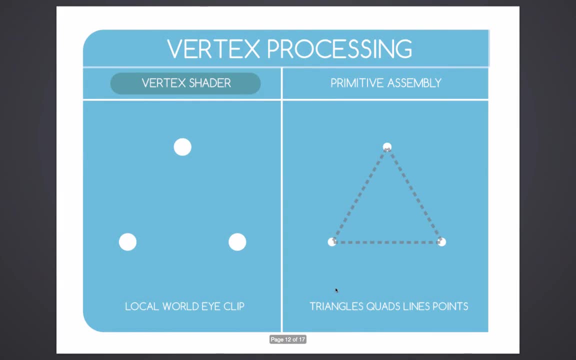 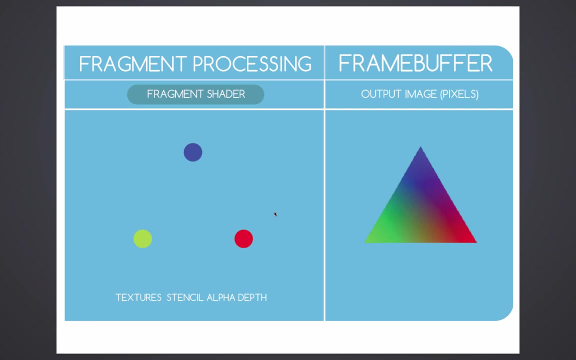 Then the pixels get a treatment called multisampling and smoothing. After we have a set of pixels driven by our data, we can now go ahead into the fragment processing. What the fragment processing is going to do- I mean, I'm sorry, the fragment shader is going to do with our pixels. 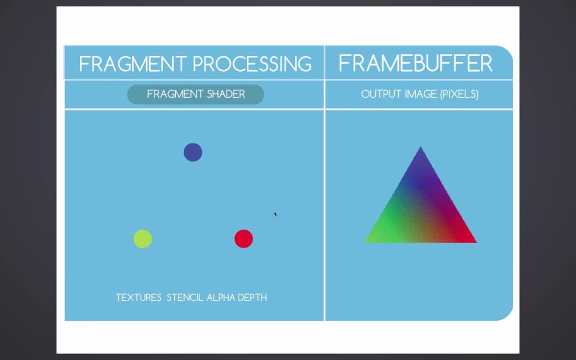 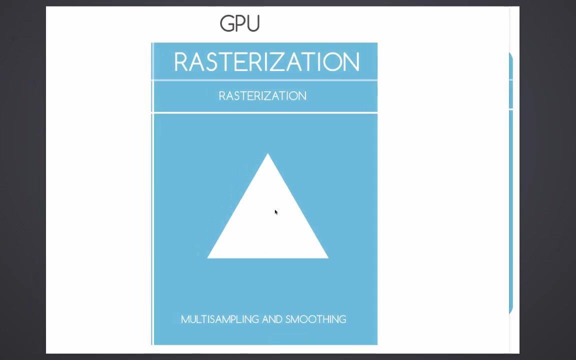 it's going to give them anything that we have established in the fragment shader, meaning textures or colors or normals or speculars, or depths or whatever we have implemented into the shader. It's going to be applied into the rasterized pixels from the vertices we have drawn in 3D space. 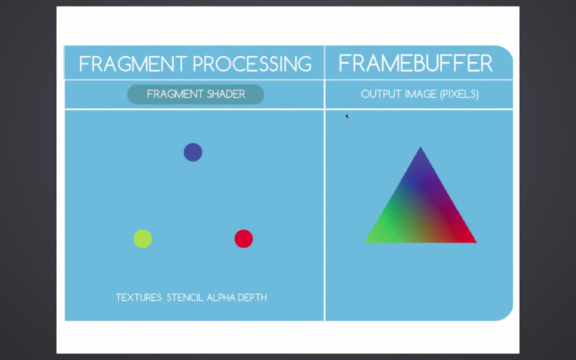 So it's getting there. It's getting there. Lastly, our fragment process. it's going to store our output, our 3D pixels, into the frame buffer. Our frame buffer is going to store the image in pixels, already with the vertex and fragment shader. 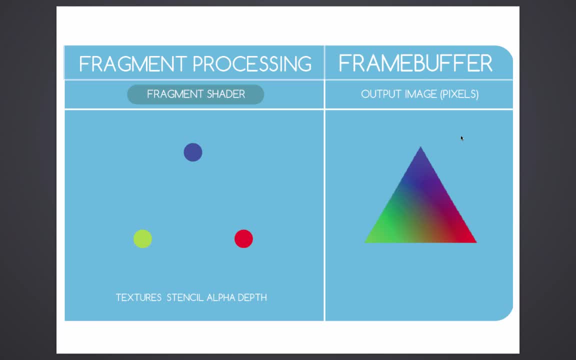 into the frame buffer. I'm sorry to be so recurrent, but I'm also understanding this graphic pipeline, So I think this step you're more familiarized with it. Whenever you're playing a game, you can check out the frames per second. 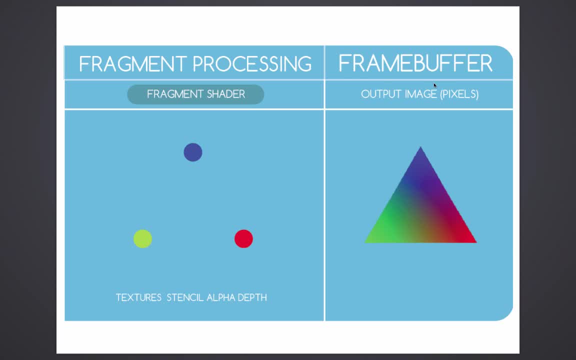 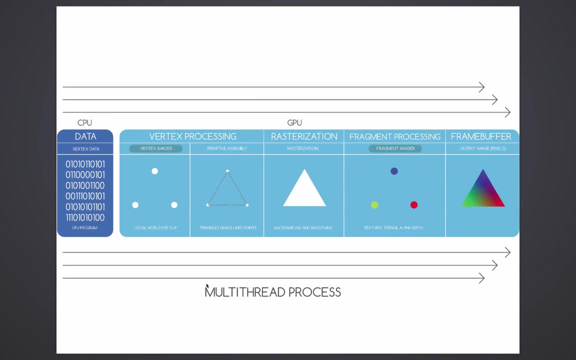 Those frames are referring to the frame buffer that is happening in the screen. This entire process. it's a multi-thread process, meaning that these all steps that I just talked about happen in parallel. They happen really fast in parallel. They do not. 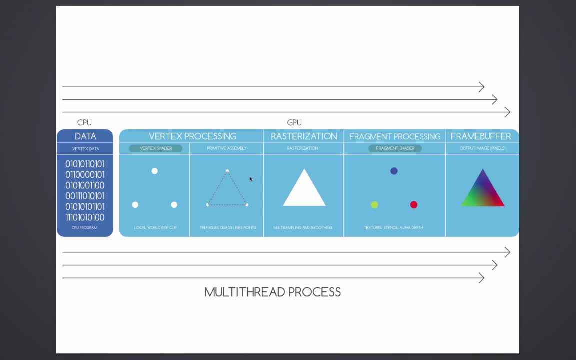 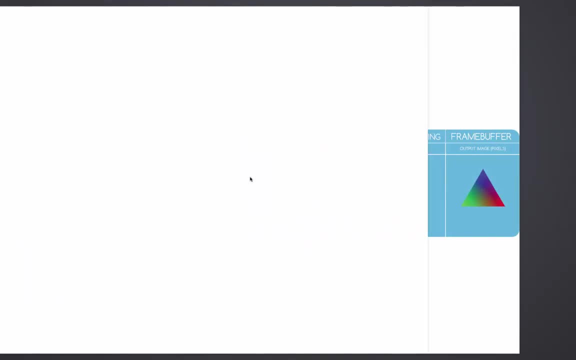 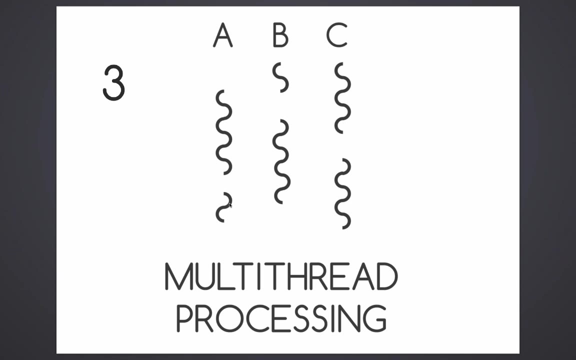 They are not linear. They're happening as we were talking- I'm sorry- As we were talking. the GPU. it's a multi-thread environment, meaning that we can have a vertex shader process while we have a fragment shader processing here. So it's happening really fast. 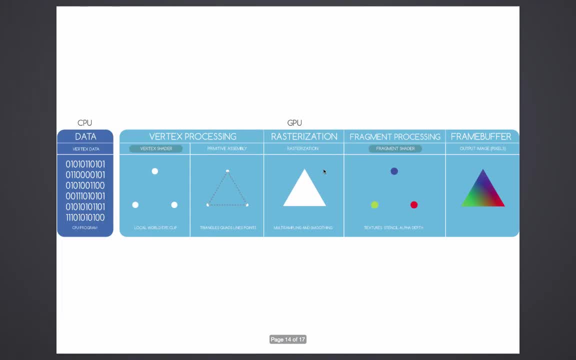 I'm speaking about millions of processes at a time, at a second. So yeah, I'm going to try to exemplify using an animation toolkit called Maya. I use it a lot to model and animate. I want to take a look at this. 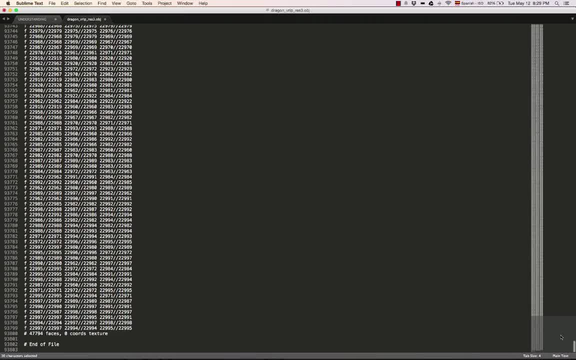 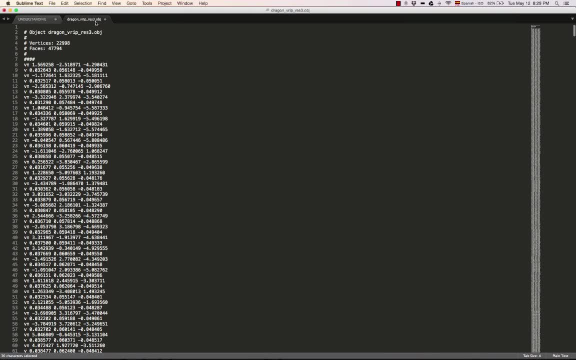 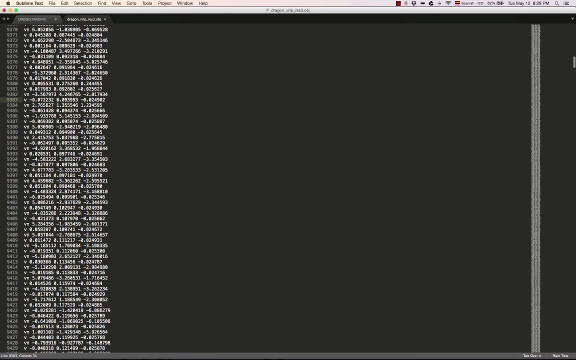 This is an OBJ file format called OBJ at Wavefront. It is a Dragon 3D model out of the Stanford 3D scan library. There's a lot of numbers here. This is a vertex and this is a vertex normal, So this. 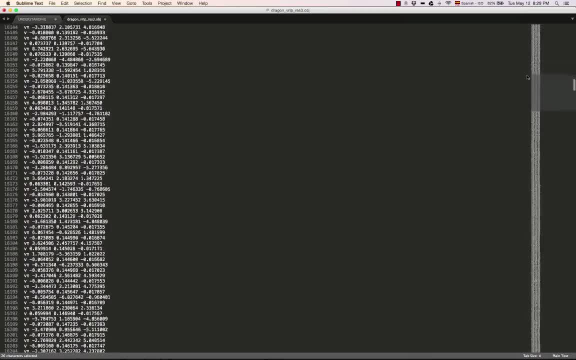 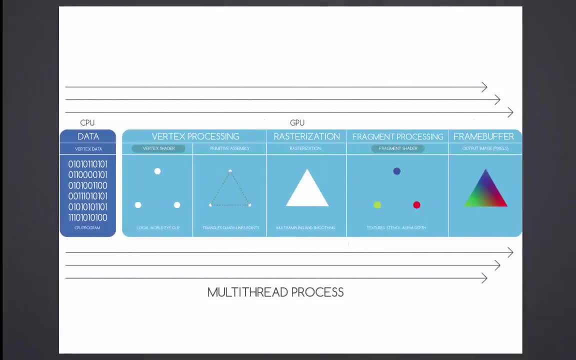 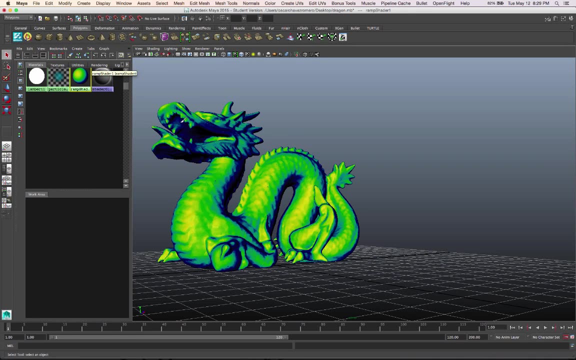 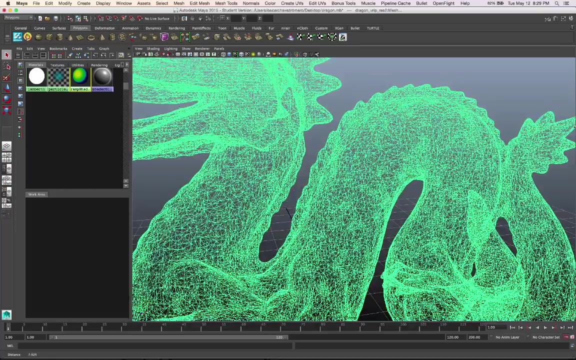 I open it with a text editor to see the incoming data, as I was talking about, And then, once you get into a rendering pipeline, you get. I'm sorry, You get this, Sorry, You get this. These are points in 3D space. 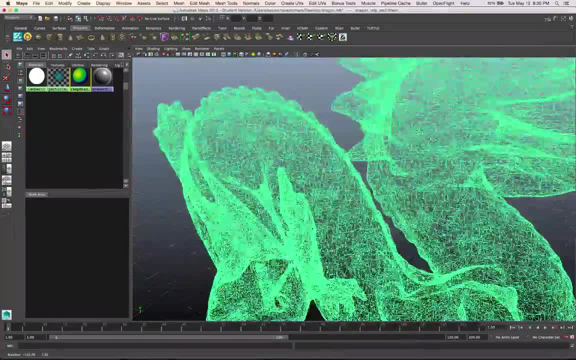 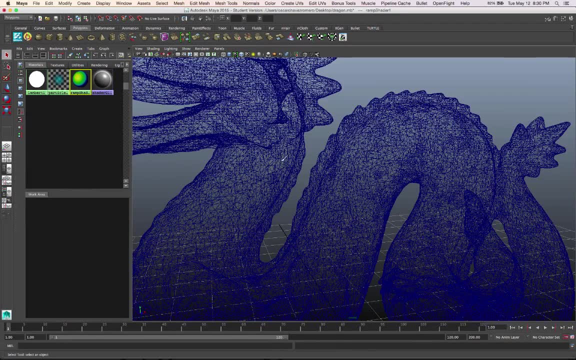 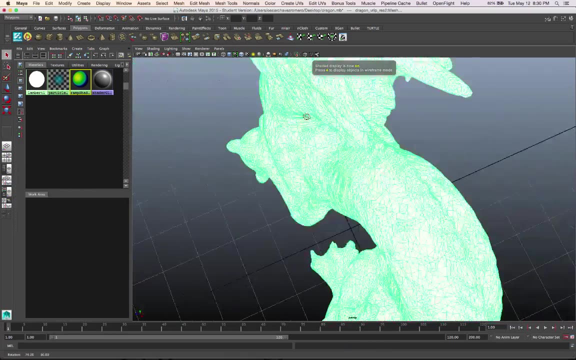 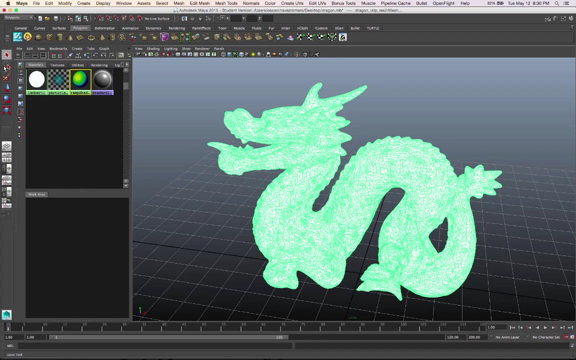 being calculated with the graphics pipeline that we just talked about. Let me get Get this. Yeah, it's being calculated. every time I rotate the camera or move it, This points are being calculated in my viewport As I speak. So, as I was saying, 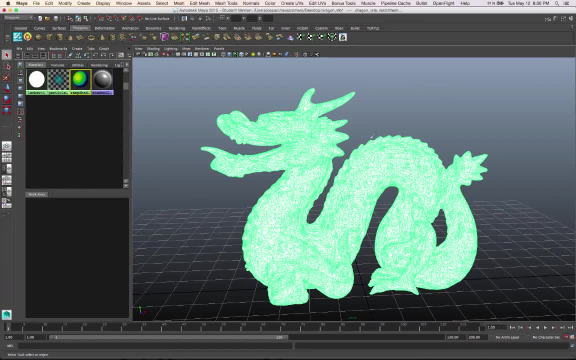 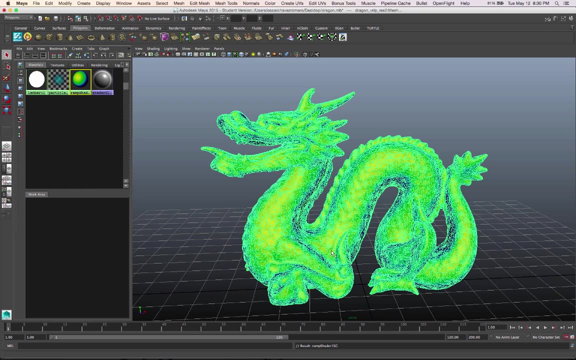 it is a multi-thread process. It takes a million, A lot of calculations, millions of calculations on a second basis And, Yeah, it finally Gives us our Oops, it's gonna crash. Gives us our fragment shader processing to render our image.